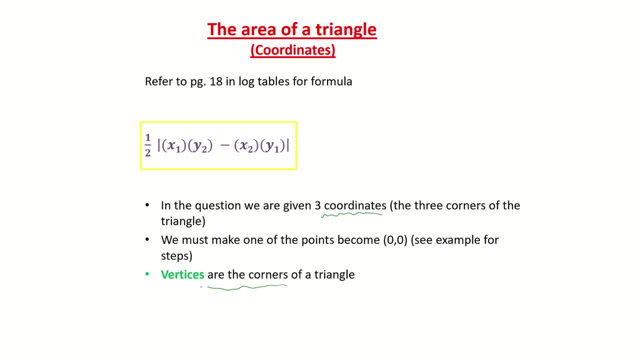 are basically the corners of the triangle, or they're also known as the vertices of triangles. So vertices just relates to the corners of the triangle. The aim of the game here is that we're going to map one of the corners to zero. zero because, as you see here in the formula, here in this yellow box, it only 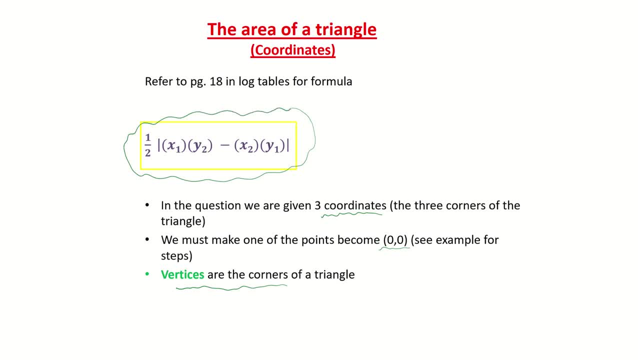 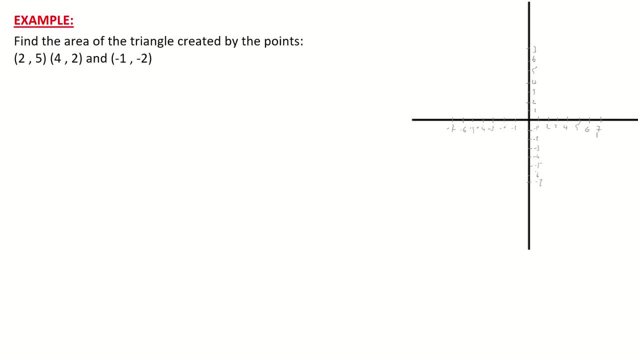 has an x1, y1 and x2 and a y2.. So you can see that there's three coordinates, but we're only actually going to use two of them, So let's have a look at an example. So this question wants us to find the area of the triangle created by the 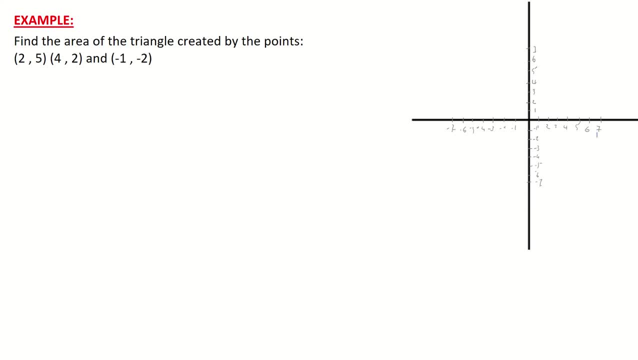 points 2, 5, 4, 2 minus 1 minus 2.. So it's sometimes useful to kind of give it a sketch first of all. So let's sketch this triangle. so our first coordinate there is 2, 5.. So again, this sketch is just to help me, or? 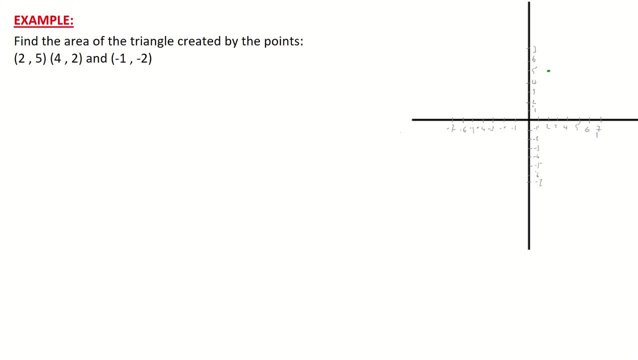 yourself visualize. it Doesn't have to be a work of art: 4: 2 and my final coordinate is minus 1 minus 2, which is down around here. Again, it's just a sketch, so I can visualize what I'm actually working with. So that's our. 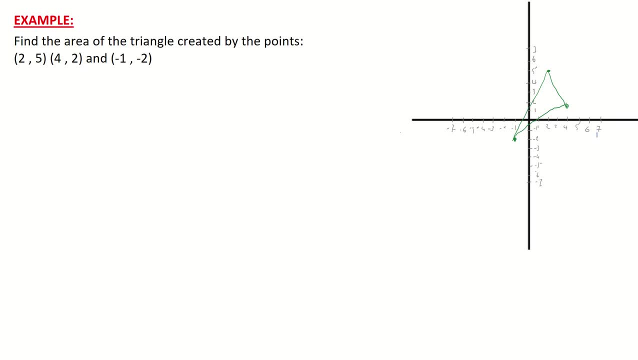 triangle. Like I said up above, the aim of the game here is to map one of those coordinates to the centre of our coordinate graph: zero, zero. Now, it doesn't matter which one you want to map to: 0, 0. It doesn't matter. So my coordinates, I'm just going to 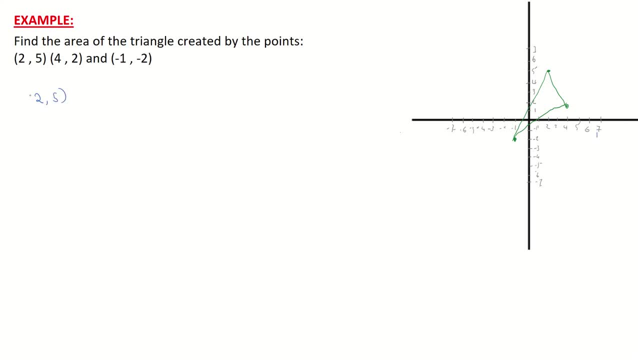 write them out. So my answer here is going to be: so: my first coordinate is 2, 5.. My second coordinate is 4, 2, and minus 1, minus 2.. And, like I said, it doesn't matter which one you want to. 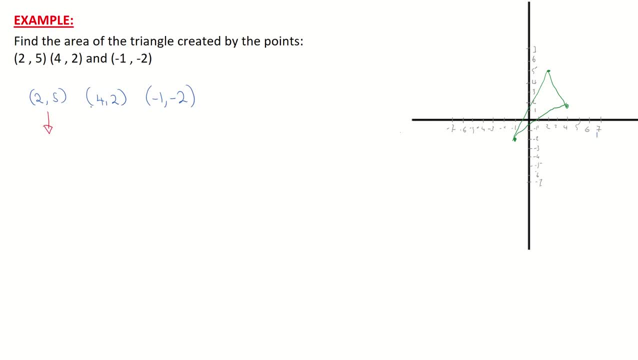 map to 0, 0.. I'm just going to work with the first one here, So I'm just going to draw arrows underneath each one. Now, like everything in maths, whatever I do to one thing, I have to do to the. 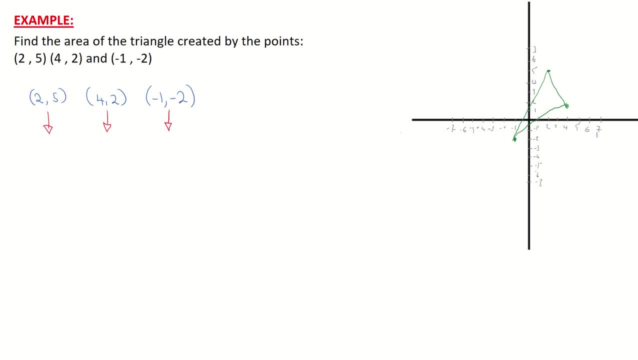 rest of them. So I'm looking here at 2, 5.. How do I make 2, 5 become 0, 0?? So if I look at the 2,, how do I make 2 become 0?? I take 2 away from it. So I'm just going to put a little minus 2 here. 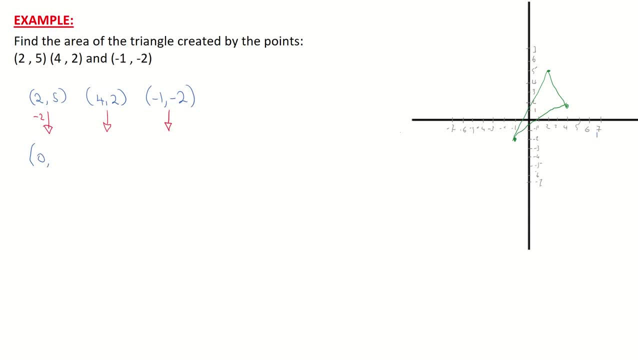 And my coordinate then will be 0, comma. Now how do we make the 5 become 0?? We take 5 from 5, because 5 take away 5 is 0. So there's my first coordinate, mapped to 0, 0.. Now I have to do the 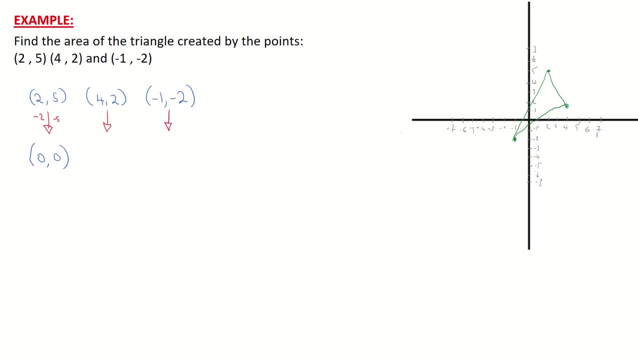 same thing here. I'm going to do the same thing here. I'm going to do the same thing here. I'm going to do the same thing to all the coordinates. So, on my x, I took away 2.. So, on my x, I have to. 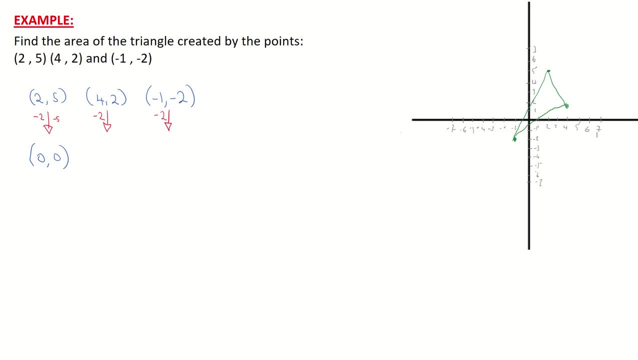 take away 2.. And on my x, I have to take away 2.. On my y, I took away 5.. So I have to take away 5. And I have to take away 5.. So you can see here that I'm being consistent: taking away 2 from. 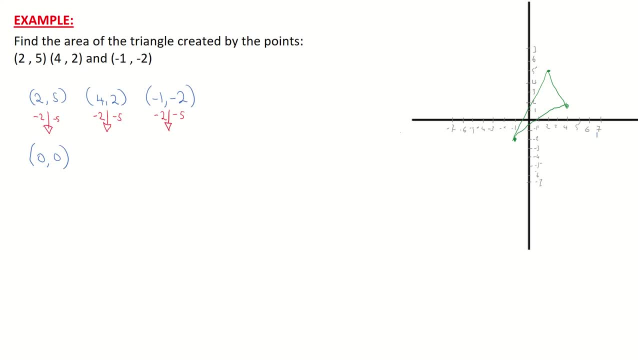 the x's minus 5 from the y's. Now, it doesn't always have to be a takeaway, It can sometimes be an addition. So just watch whether you're trying to add to get to 0 or take away to get to 0.. 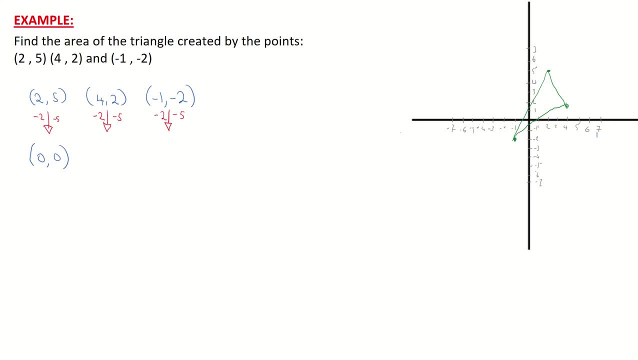 Now, when I finish out my other two coordinates, what's that going to give me? 4, take away 2 is going to give me 2.. So that's the x on my coordinate, And then I'm going 2, take away 5.. 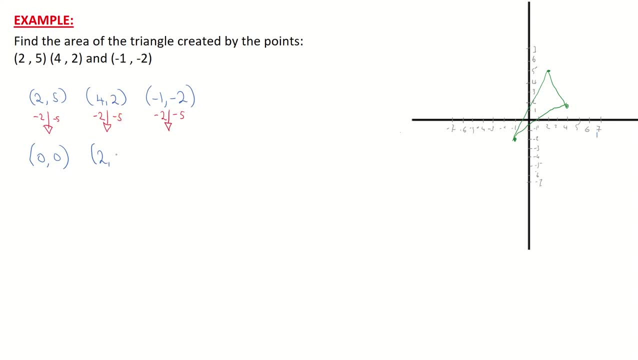 2 take away 5 on my number line is bringing me to negative 3.. I'm then coming to my final coordinate, And it is minus 1, take away 2, which is bringing me to minus 3.. And I have minus 2, take away minus 5, which is bringing me minus 2.. Take away 5 is bringing me. 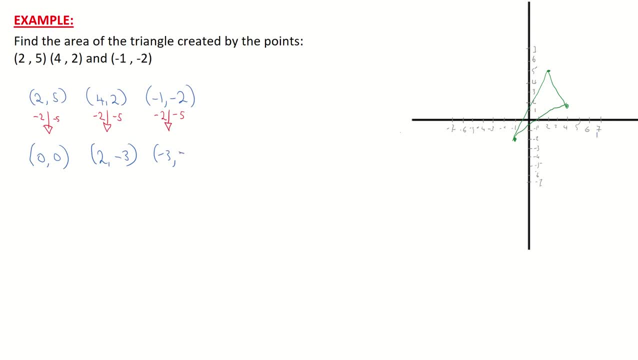 to minus 7.. Okay, So you can now see that we have our three coordinates And I have 0,, 0,, 2, minus 3, minus 3, minus 7.. Again, I'm just going to come over here and sketch that just for myself. 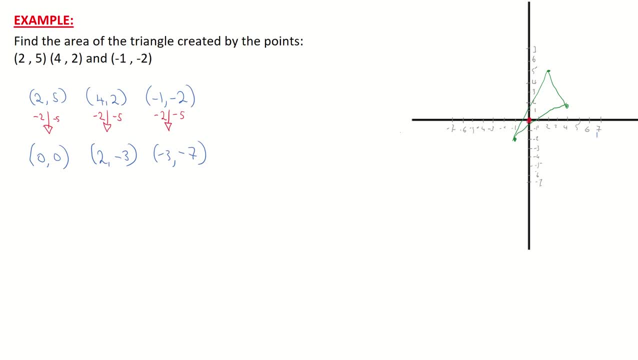 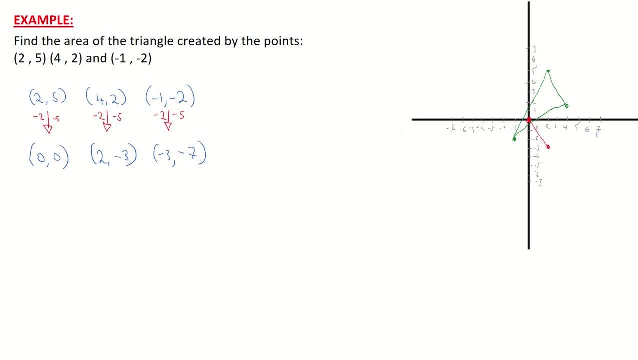 3,, which is down around here, And I have a minus 3, minus 7,, which is down here. So you can see that all I've done is basically moved my triangle. It's still the same shape and same size. All I've. 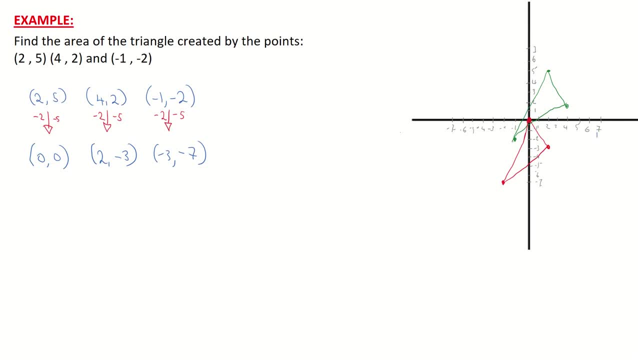 done is basically moved it from one position to the other. So you can see here that these corners have been mapped. You can see that I'm just basically moving my triangle across my coordinate graph. Okay, So, coming back to my three points, I only have to work with 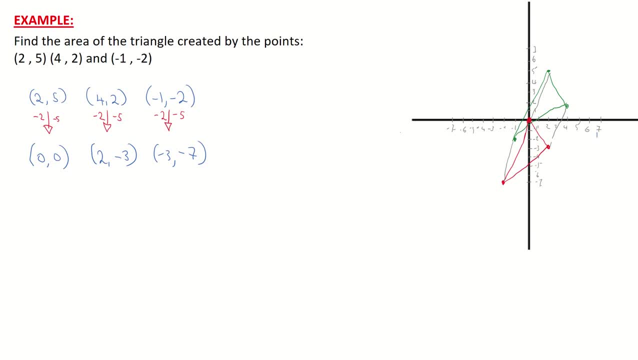 two of these points here. now, of the three, You always ignore the 0, 0. So I'm just going to put an x through the 0, 0.. I'm now finished with that coordinate. I don't work with it anymore. 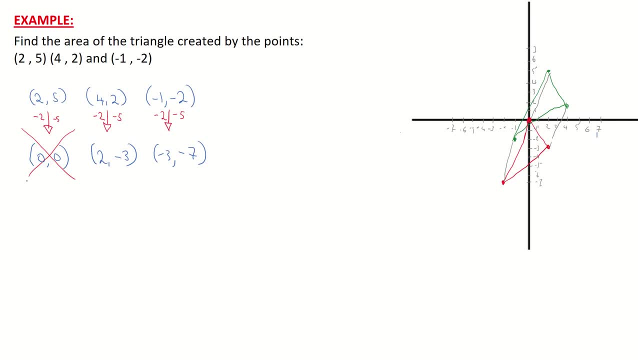 With my other two coordinates. I'm now going to label them x1, y1, and x2, y2.. Now it doesn't matter which coordinates you call x1 and y1 and x2 and y2.. Just be consistent. And now I'm going to fill those two coordinates into my formula. Now, 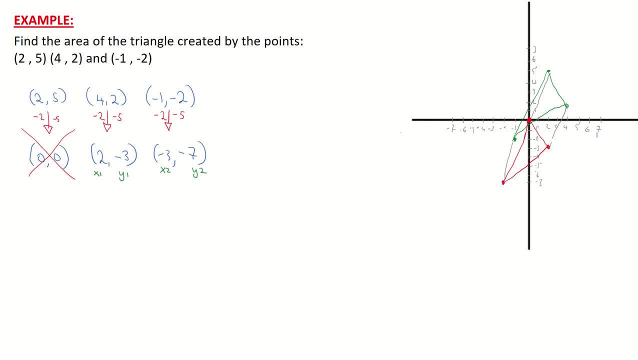 my formula for the area of the triangle is x1, y1, and x2, y2.. So I'm going to fill those two coordinates into my formula. Now my formula for the area of the triangle, when I'm given three coordinates, is half x1 times y2 minus x2 multiplied by y1.. Now that formula is in your log tables. 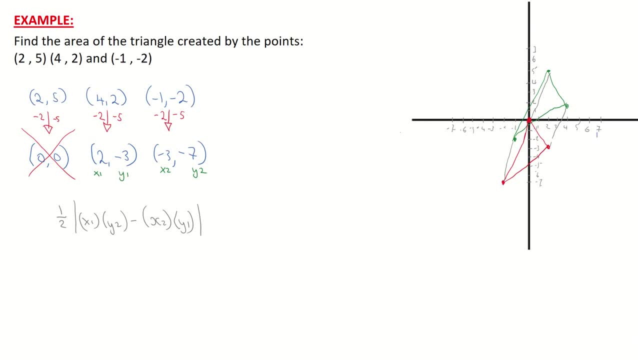 And a couple of things we're just going to look at here. It's always half, because it's half of a rectangle for the area of our triangle. These square brackets are absolute values, So that basically just means nothing complicated In maths. basically the formula is getting us an area. 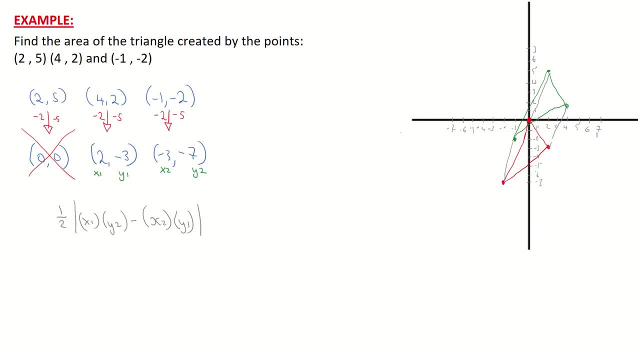 of a triangle, which may be a negative answer, But we know in reality that the area of a triangle must be positive because it's the area. So it basically just means we turn our answer into a positive answer And filling in our formula. So what does that give us? So we have half bracket. 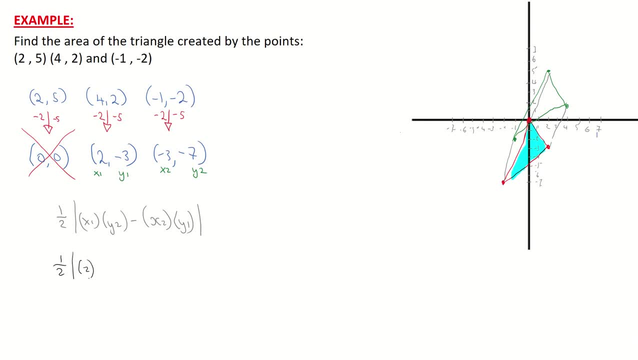 x1.. Now our x1 is 2.. So again, I'm going to just put that into a bracket: multiplied by y2, which is minus 7.. So just be careful here with the signs and your brackets. And now, subtracting x2, which is negative, 3: 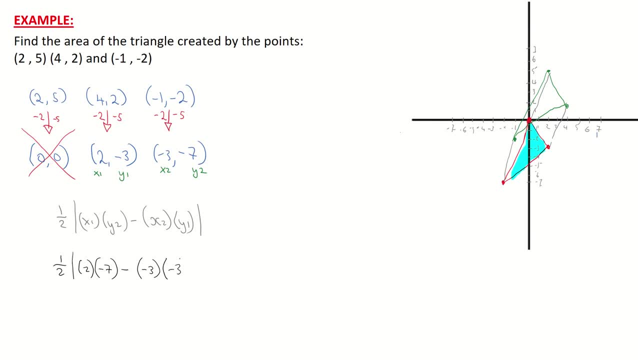 multiplied by my y1, which is also negative 3.. It just happens to be the same in this question. So that's giving me a half bracket. 2 multiplied by minus 7 is giving me minus 14.. So I'm just.